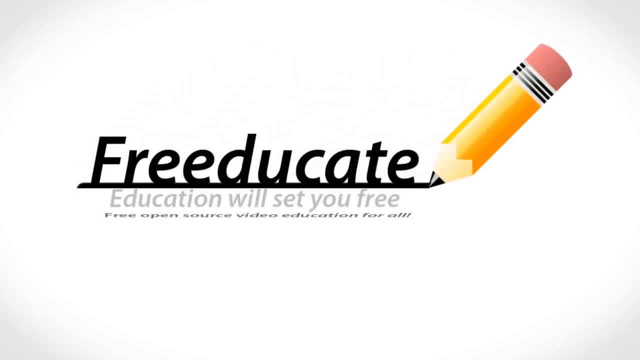 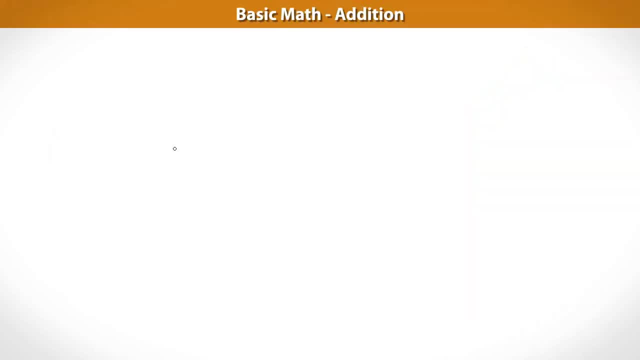 Welcome to this video on basic addition. If addition is not basic for you, no need to worry. You'll be up and running in no time and adding real numbers. So, what do you need to do in order 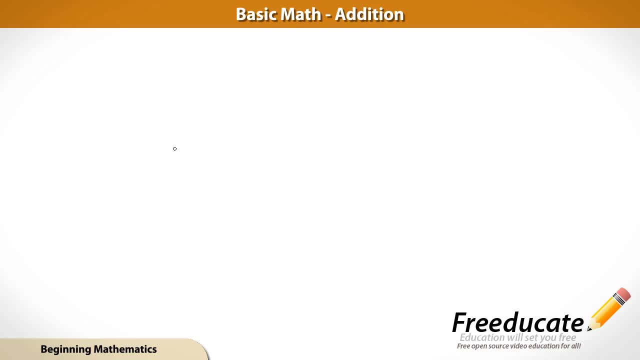 to add and use basic addition? Well, the most simplest form is a 1 plus 1 equals 2. If you relate this to the real world, that's like one object plus another object equals two objects. And the objects can be anything. So, let's take a look at how this works and you'll get a better feel for it. So, if we have 1 plus 1, that's going to equal 2. So, it's pretty straightforward. You 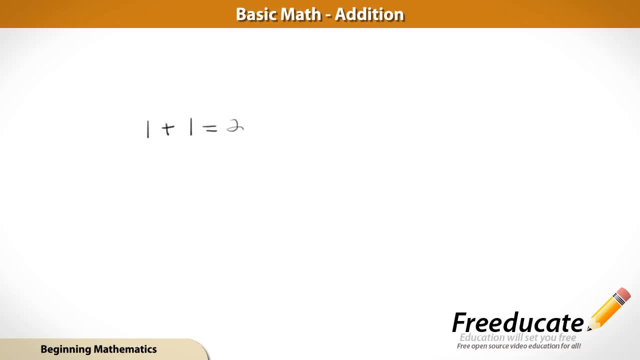 have one object. Actually, let me go ahead and make this a little clearer for you. You have one object plus another object equals two objects. So, pretty straightforward. It's like if you take yourself as an object and then you're hanging out with your best friend, that's another object. You both are people, but you're also objects. So, one person plus another person equals two people. Very simple. Straightforward. Let's relate this to the real world. If addition is not basic for you, no need to worry. 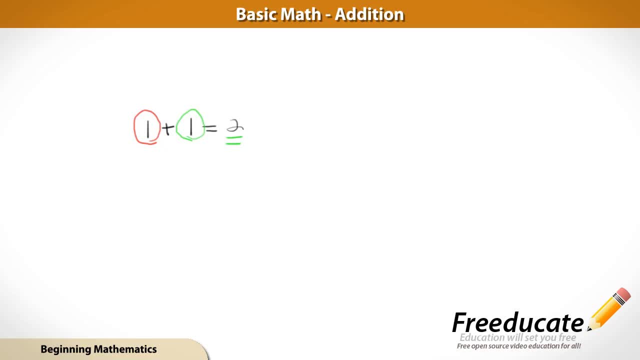 You can use this to, let's say, apples. If you're going to the grocery store and you're real hungry and you pick up one apple and then you decide, you know what, I'm even hungrier than I thought, and you pick up a second apple, that's going to give you two apples. Again, this being one object, this being another object, and then ultimately, 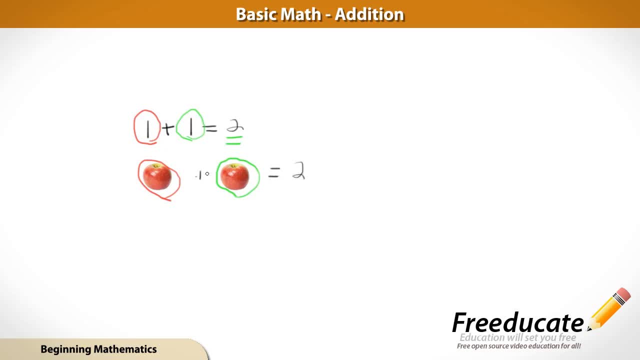 equals two. So, you have one apple here plus another apple here equals two apples. All right. Now, what happens if it's always not a one-to-one type of situation? What about if you, say, you decide you're not really a big fan of red apples today and you decide, I'm liking green apples, and you go with four green 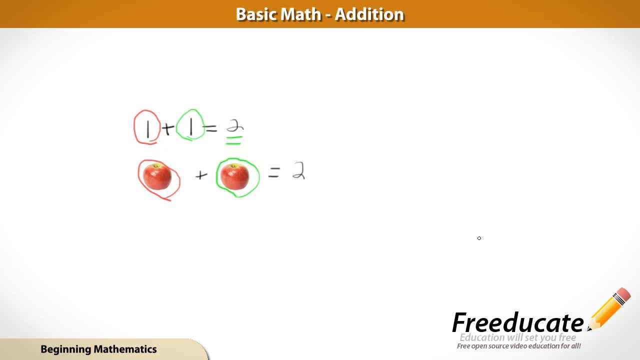 and three red apples. So, you go with the simple addition of four plus three. Well, that's pretty easy, too. Let's take a look at how this works. So, if we come and we look, you're going to see that we have four apples plus another three apples is going to give us how many apples. Well, what you could do, you could do something real easy. You could count how many apples that you see on the screen. You could go one, two, three, four, five, six, seven. So, now, you know you have seven apples. So, the problem 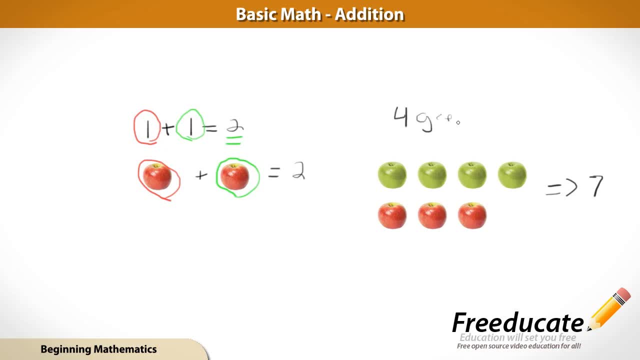 would look like this. It would look four green apples plus three red apples. 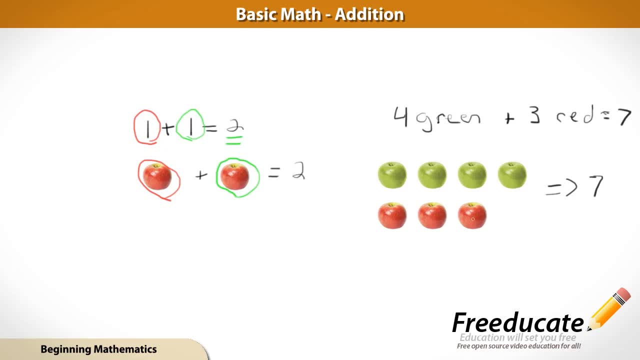 That equals seven apples. Again, very simple, straightforward. I'm going to write this a little bit neater for you. So, this comes down to four plus three is equal to seven. All right. Now, if you want to actually relate this to something like, let's say, a number line and get rid of the real-world objects, this is really easy to do, too. 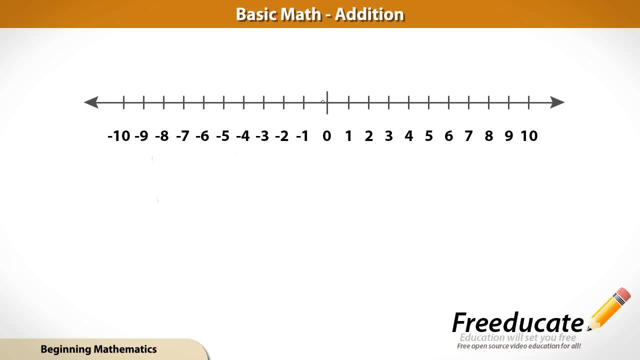 All you're going to be doing on a number line is you're going to be hopping. You're going to be starting at your first position and then hopping to your next position. And, as always, what we do on a number line is we start from zero, or we start from the number that we're working with, and you hop what the other number is in whatever direction. So, let's just go ahead and see how this works, and you'll get the hang of it. Right now, zero is always home base, so to speak, but let's say we had our green apples, and we had four green apples, and then we had three red apples. So, in order to get to our red apples and get our total number of apples, we're going to hop three spaces. So, we go one, two, three. So, we have four green apples, hop three times on the number line, and that's going to give us seven apples. So, now we have seven apples in 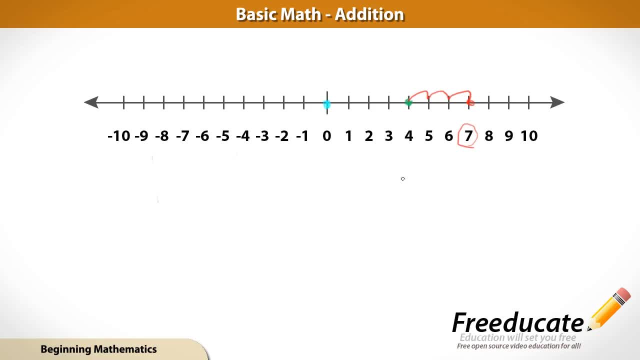 total. Now, also, let's think about this if it was backwards. Let's say we had something like, three, plus four instead of the four plus three that we just did well you can do this the exact same way let me go ahead and clear this and what you're going to see is now if we go with our red apple or if we go with our red apples instead of our green ones first we start out 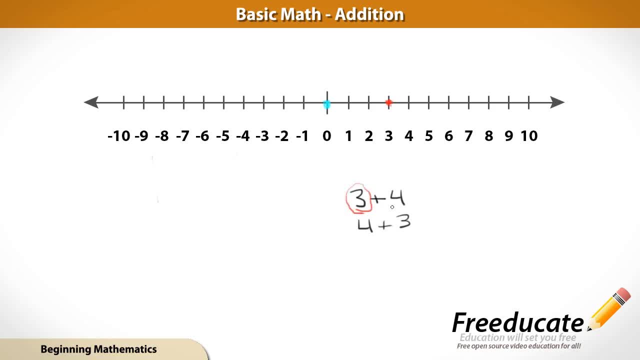 at three because start out with three right here and then we go add four more to that so we hop on the number line one two three four times and we end up right here 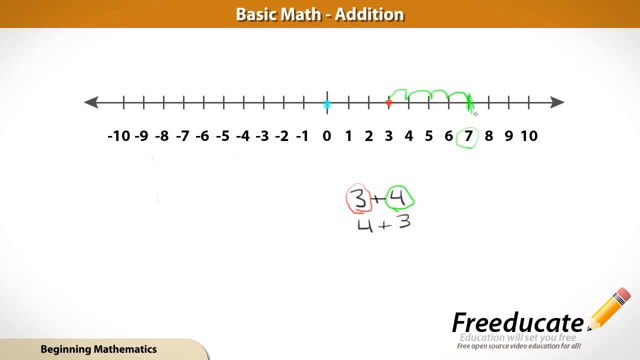 again we still have seven apples so no matter which way you do it which number you start with in addition it's always going to be the same this one is equal to seven 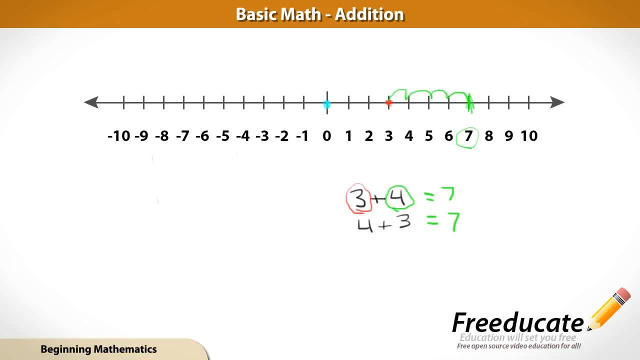 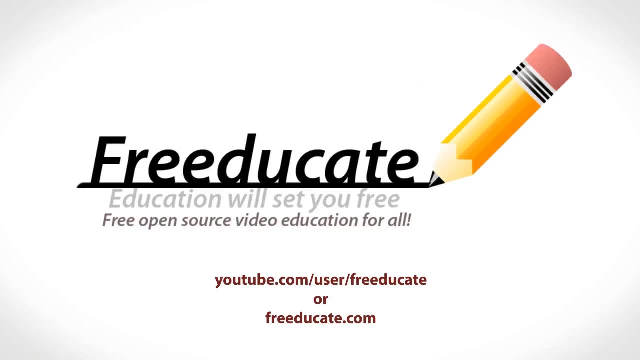 as this one is also equal to seven so again this is very straightforward process nothing terribly difficult about this if you need more help feel free to visit us at youtube forward slash user forward slash for educate or visit us at freducate.com for more conversations and information into its basic edition again i appreciate your time we'll see you next time What are acids and bases? 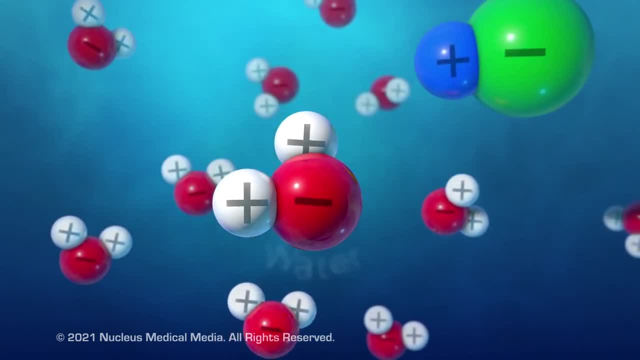 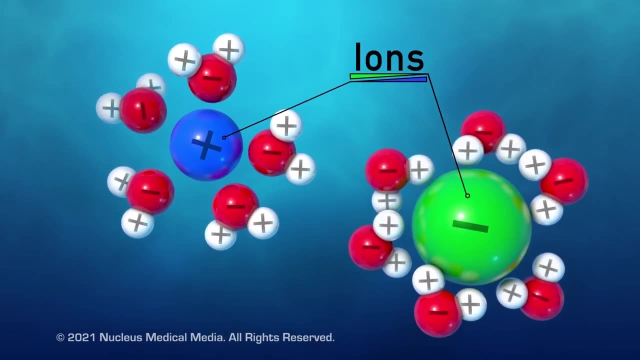 First, recall that water is a polar molecule that dissolves ionic compounds by separating them into negatively and positively charged ions. 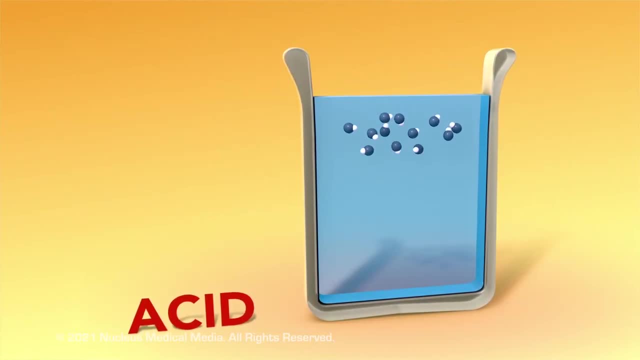 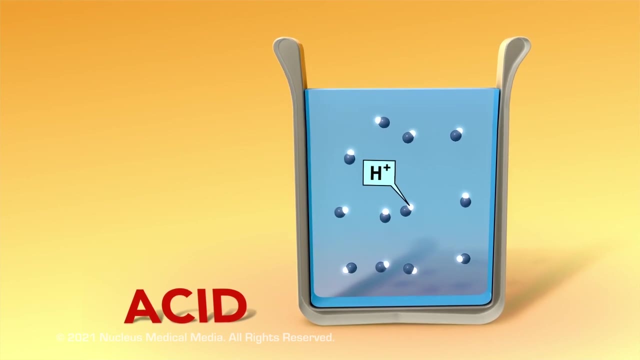 An acid is an example of one of these ionic compounds. A sample of this type of substance contains an abundance of positively charged hydrogen ions that are released from the compound when dissolved in water. 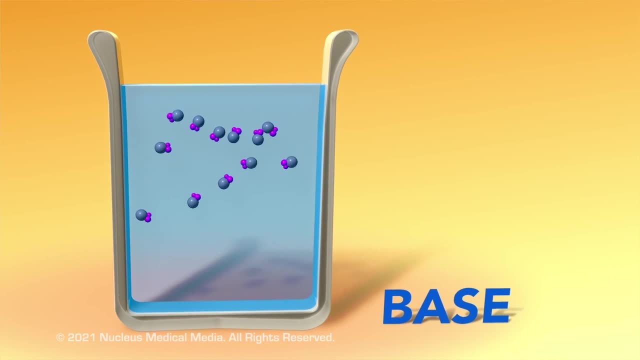 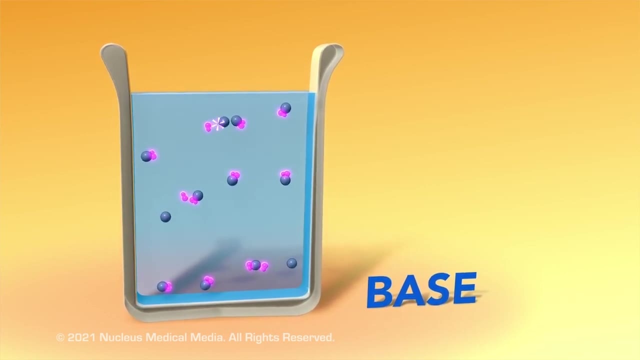 A base is also an ionic compound, but a sample of this type of substance contains an abundance of negatively charged hydroxide ions that are released from the compound when dissolved in water. 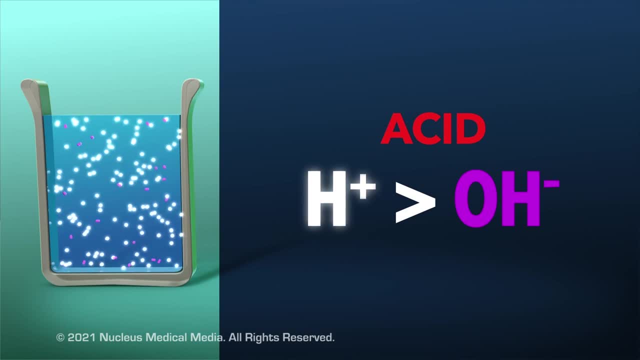 An acid always has a greater concentration of hydrogen ions than hydroxide ions. 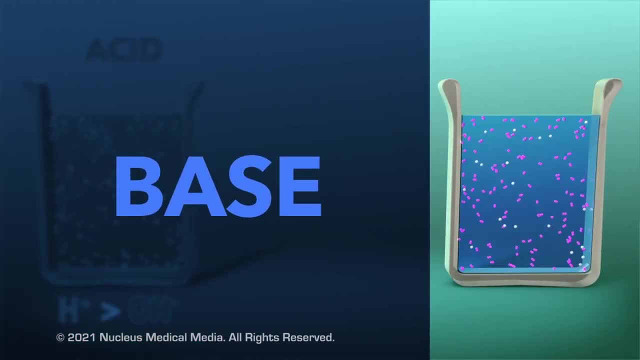 In contrast, a base always has a greater concentration of hydroxide ions than hydrogen ions.